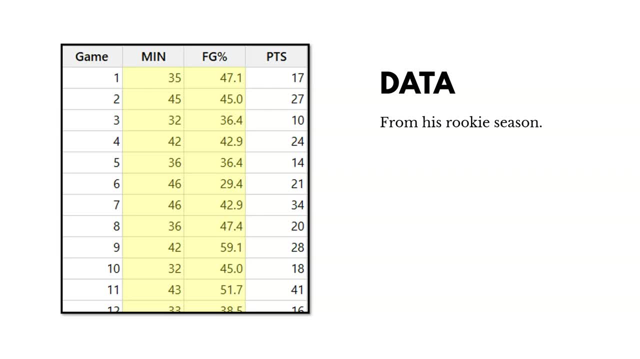 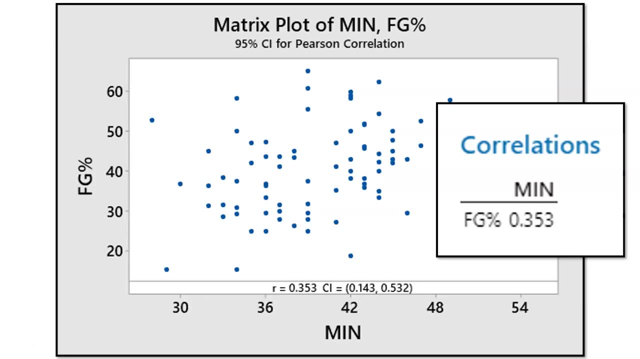 So his field goal percentage is based on how many times he shoots it, what percentage does he actually make a basket, And so I use a tool called Minitab to do this, but you can use Excel or other tools. But once I do that, I'm going to get a scatter plot like this and a correlation coefficient. 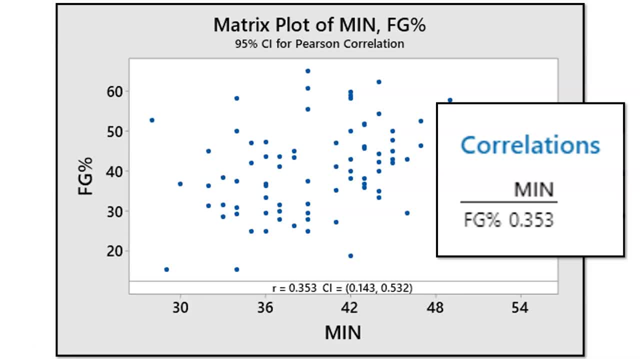 So on one axis we see his minutes per game And another we see the field goal percentage, And every data point represents a different game And we can tell by looking visually at the scatter plot, but also by looking at the correlation coefficient. 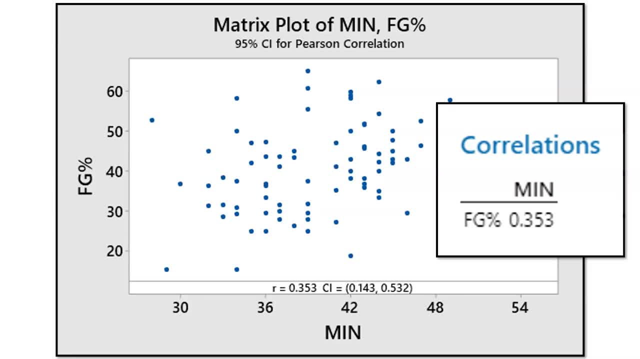 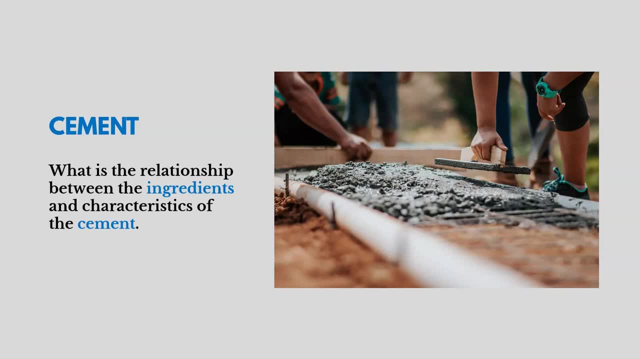 that it's a positive relationship, but it's somewhat weak- 0.353.. Now let's take a look at another example. Let's think about cement, And maybe we want to understand the relationship between the ingredients of the cement and characteristics of it. 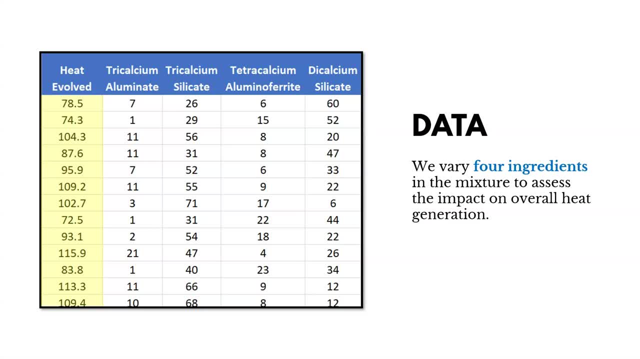 And so we gather data like this: We vary four ingredients in the mixture to assess the impact on overall heat generation. And so on the right-hand side here you see four ingredients of the cement. On the left, you see what's called heat evolved. 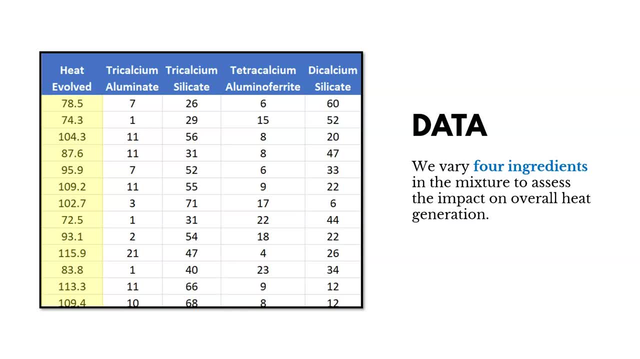 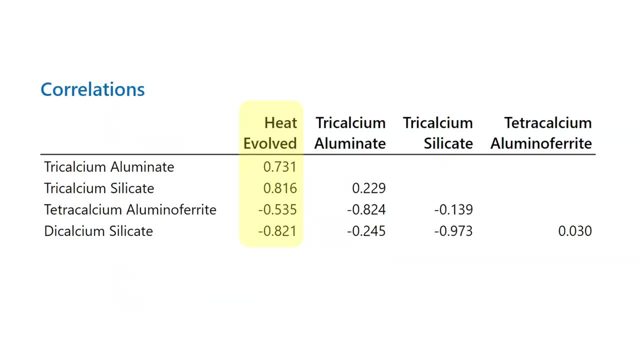 We want to understand how these ingredients are related to heat, evolved a measurement or characteristic of the cement, And so we can generate, in this case, a correlation matrix, because we have more than two variables And what you see highlighted here is the correlation coefficients. or the relationships between the ingredients. On the left we have a correlation matrix, And on the right we have a correlation matrix, And on the left we have a correlation matrix, And on the left we have a correlation matrix And on the left we have a correlation matrix. 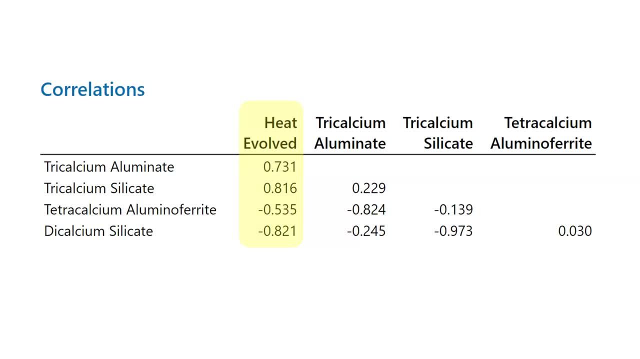 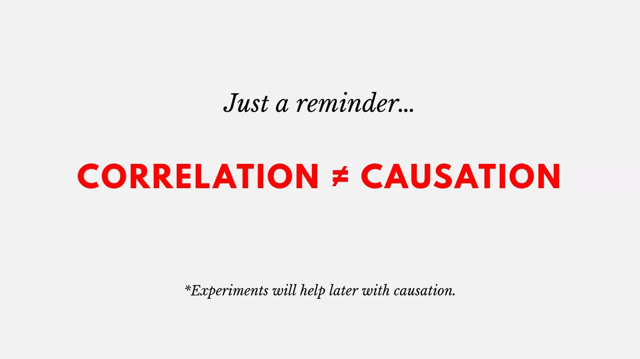 And heat evolved, So two of them are fairly strong. positive, So as the ingredients go up, heat evolved tends to go up as well, And the other two are negative, So as the ingredients go up, heat evolved tends to go down. Now, one thing to remember as we finish here is that correlation is not causation. 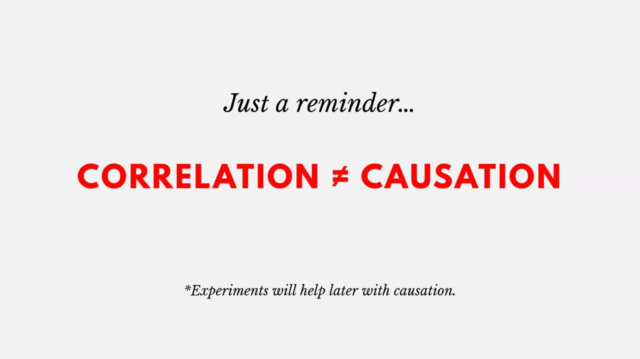 So just because there's a relationship in how they move, it doesn't mean that a change in one is causing the change in the other. So there's correlation but not causation, necessarily that they don't equal each other. So experiments can be used to help us later with causation. 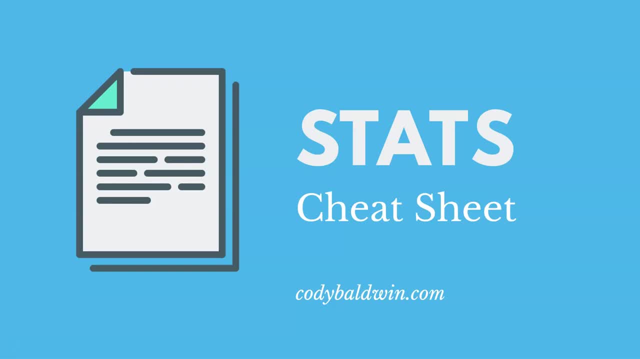 Thanks for watching. As a reminder, if you want a free stats cheat sheet, you can find one at CodyBaldwincom.